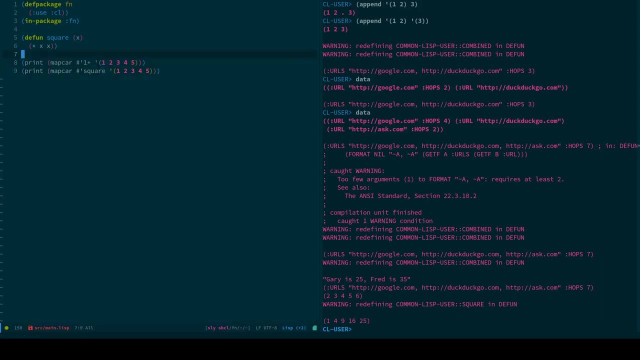 using the square function. Now we can extend this and we're going to have a look at reduce, Where map car takes a list and gives us a list of exactly the same length. back. reduce takes a list and does something with each of the values, accumulating them or folding. 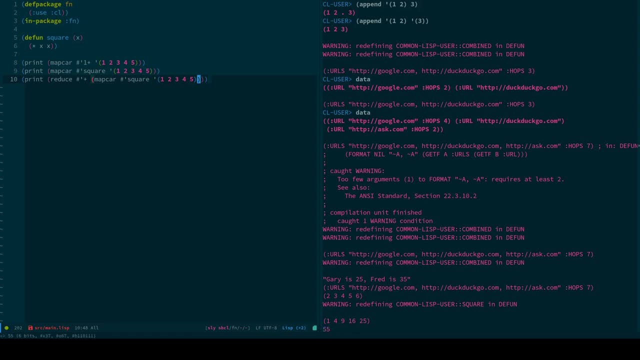 them together to give us one value. So here, where we map, car over the list of squares and we're basically just summing the list of squares, we get 55, which to prove that that's totally not what I wanted to do there. There we go, We still get 55.. So these two 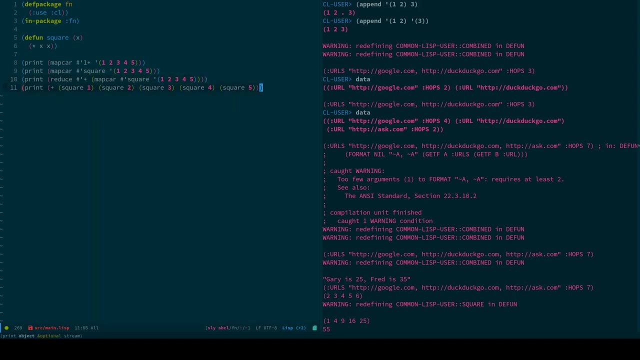 lines 10 and 11 are equivalent to one another, 10 hopefully being significantly more readable to you. So that's how map and reduce work together, And I appreciate that this is really a very small example. So we're going to have a look at how to introduce more complexity, And I'm 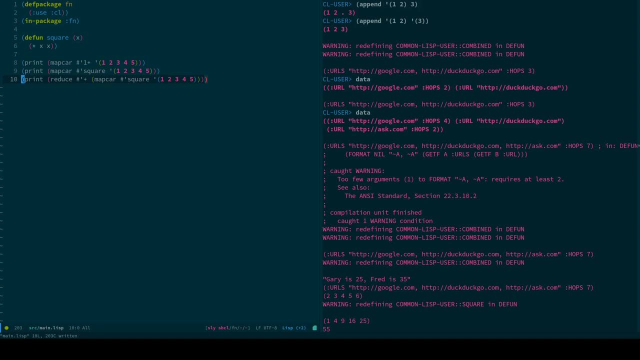 going to pull an example that I worked on something similar in a previous company, just with all the sensitive stuff stripped out of it. So let's have a look and build up our understanding here. One of the things that I wanted to look at in previous videos that I wasn't thinking. 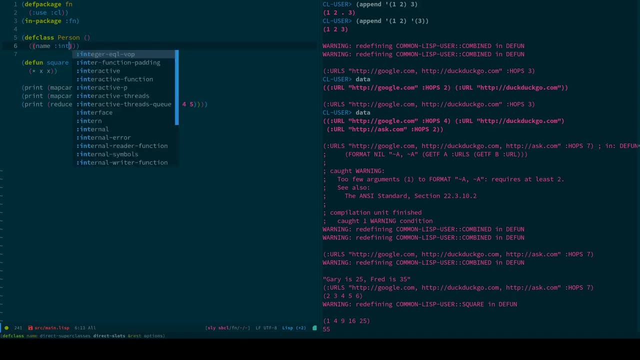 is. I want to show you how we can use class here. I'm just going to have our class here. There we go, and we are going to add in a method for printing this out. so I'm going to say defmethod, I'm going to say print object, and this takes a object which is person, and it takes a stream. 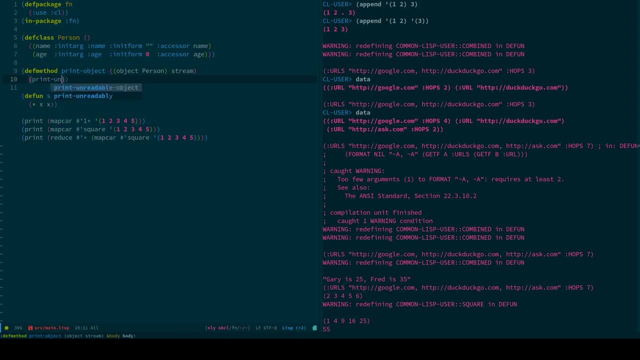 and we're going to say print readable object, which then takes a stream and that then formats the stream. let's take a and then we're going to say main object and age object. so that's all balanced out there, Just because that's always easier to work with. 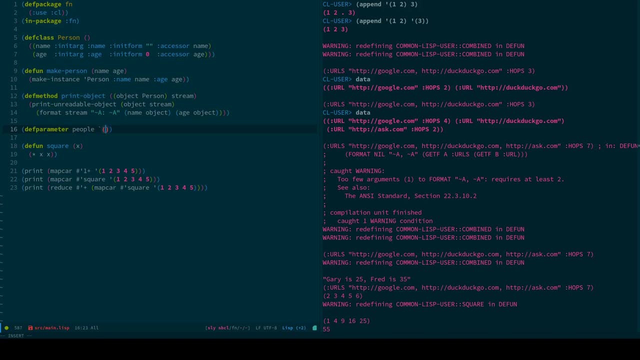 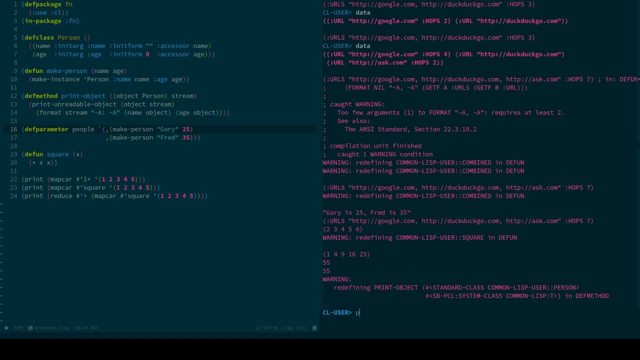 So one of the things that- So one of the things that You have to make sure that you're doing- Is that you're using the back ticks To do that. we want to make sure that we've got our objects here if we didn't use the 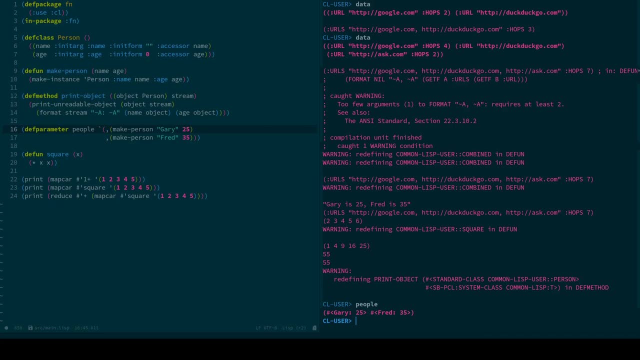 back, ticks, Commas. we'd end up with a list of symbols that represented the code to build up an object, but not actually the object itself. So when you're wanting a list of objects and you want to make sure that you are, 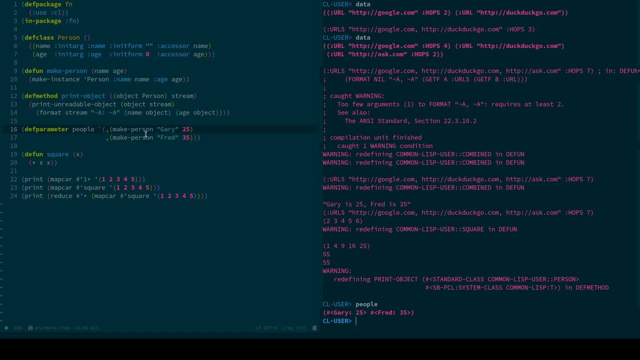 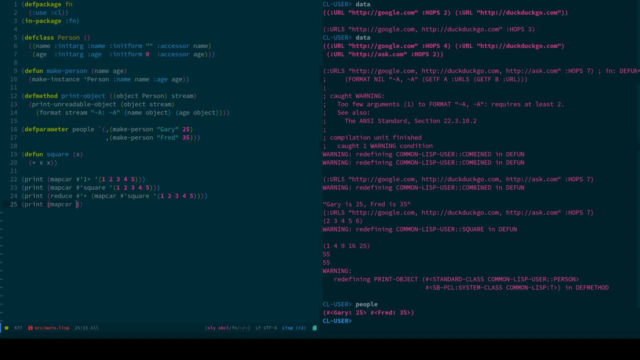 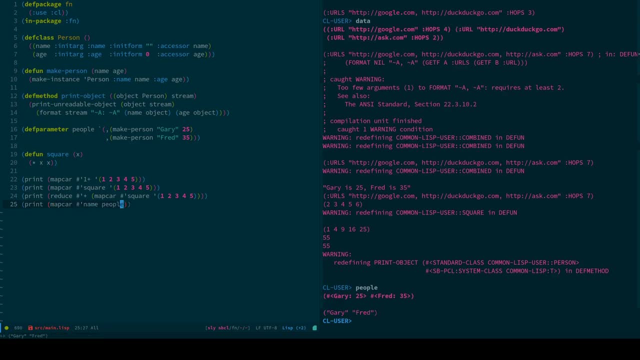 So here we give over 2. We use the age, we get 25 and 32.. So we can easily plug Kloss into this, as long as we are again using the right form. here We use the age, we get 25 and 32.. 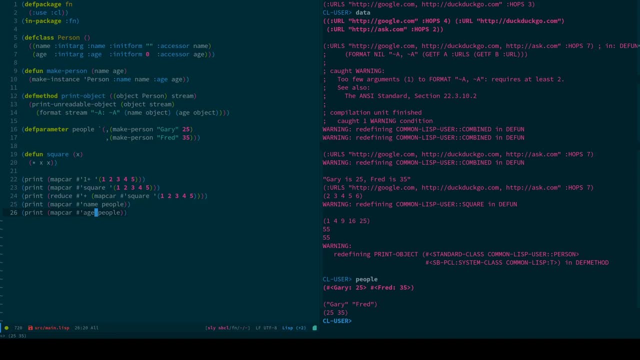 So we can easily plug Kloss into this, as long as we are again using the right form here. Now we might want to define a function. There we go, There we go. so we've got this pretty printing thing here and we are going to. 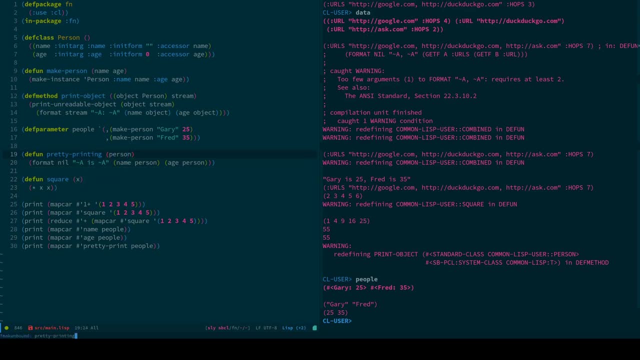 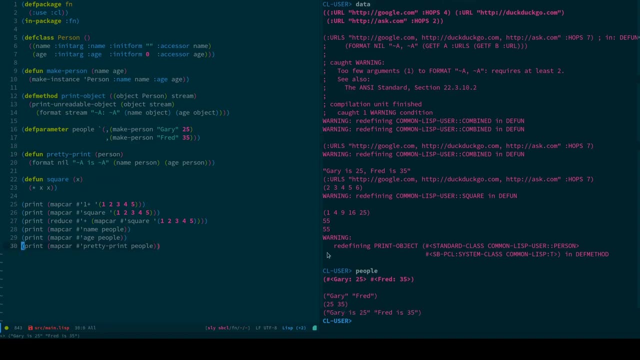 Pretty print, not pretty printing. There we go. So we get this list here of Gary is 25,, Fred is 35. Now what we're going to do is we're going to write a join method which takes an A and a B. 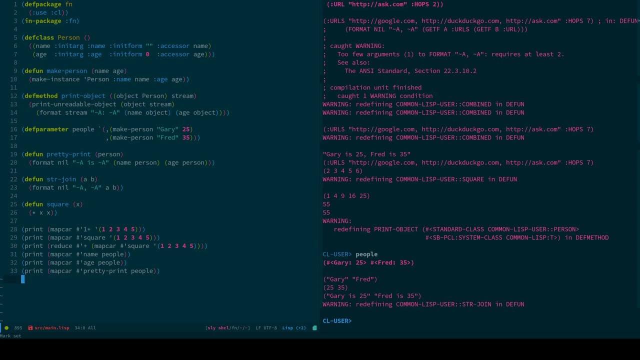 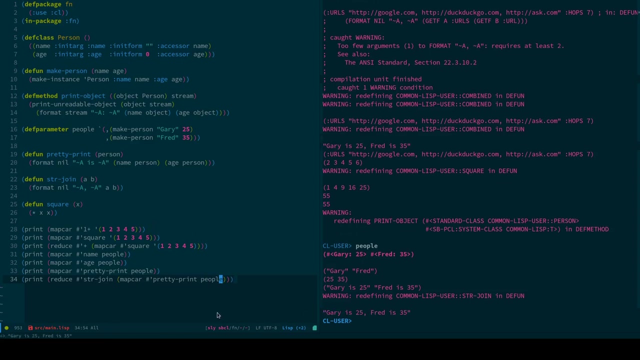 There we go, There we go. So, now that we've got all this in place, now if we print out the result of reducing by string, join the map condition. So in the case of a car of pretty printed people, we get: Gary is 25, Fred is 35.. 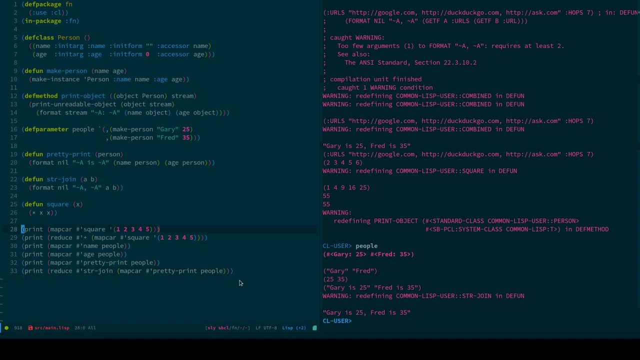 So let's clean this up a bit with some of our trivial examples here. There we go. Now this might look like a very simple example, So what is going to follow in the next few minutes is I'm going to try and build up. 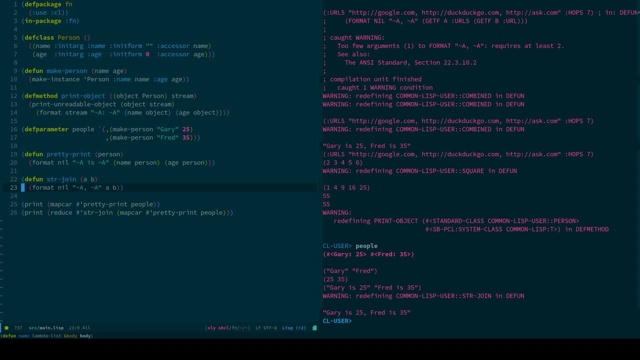 A slightly different example and I'm going to build up a list of data, and it's just going to be a list of URLs and hits. Be aware that these numbers are in no way going to be anything close to realistic And be aware that I have omitted this. hits here from this second, deliberately. 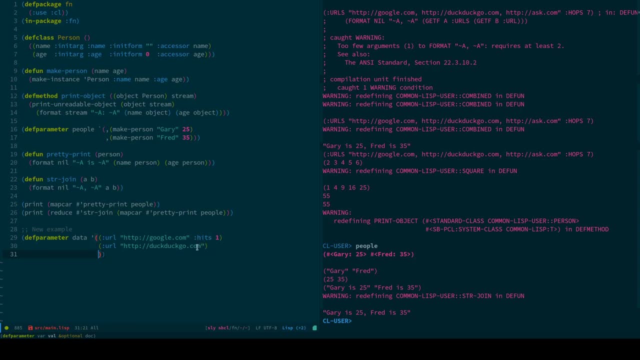 We're going to treat this record as if it is missing some data. It's been a while since I've seen Q. that went away many years ago, And let's stick with defunct search engines. I guess There we go. so if we print this out, we'll see that we've got a list of items here, three. 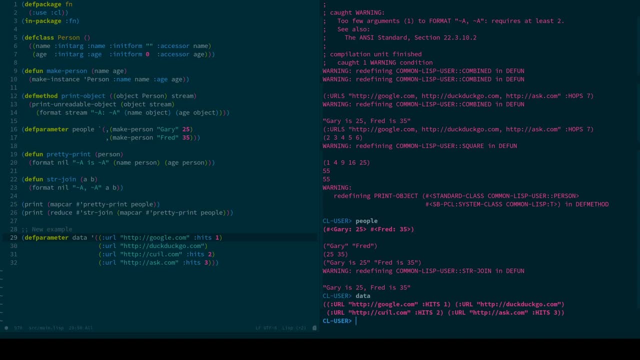 have this hits thing. The second does not. So what we need to do- and this was based on a bug in some real software that I was working on about a year or so ago- the front ends, the JavaScript front end, if a user failed. 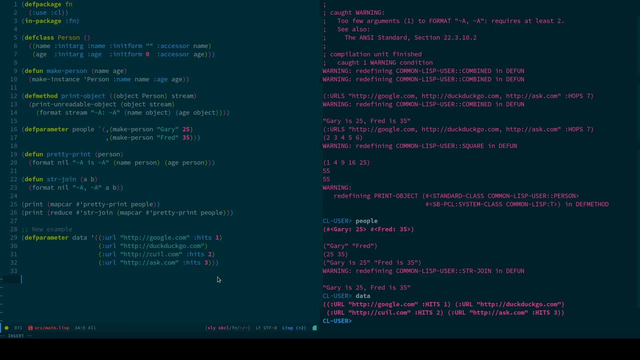 to click the appropriate box, JavaScript would sound like undefined and then our backend would parse that as being like zero or omit it and just not build up a dictionary or an object hash map correctly And we would have bugs where things wouldn't have the appropriate bits of data. 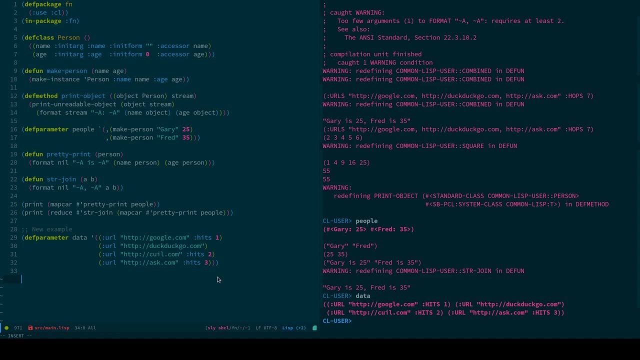 So this is a down. I've taken all of that away, and it wasn't even written in Common Lisp, but this is based on a real flaw that we had. So what we could do is defunct, fix missing hots. then this takes an object. we say: if 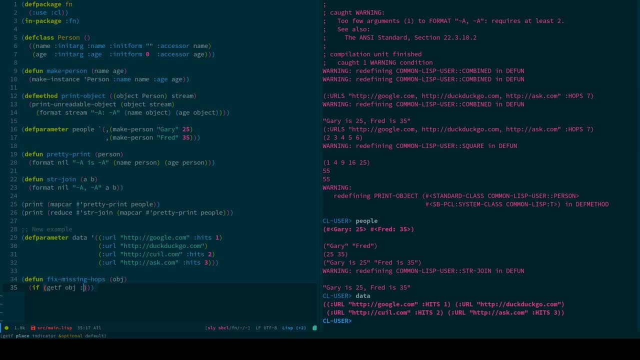 get object hits, fix missing hits. So if it does have that, we're just going to return object. otherwise, we're going to return a new list which is going to contain and hits. so that's going to be a new list. 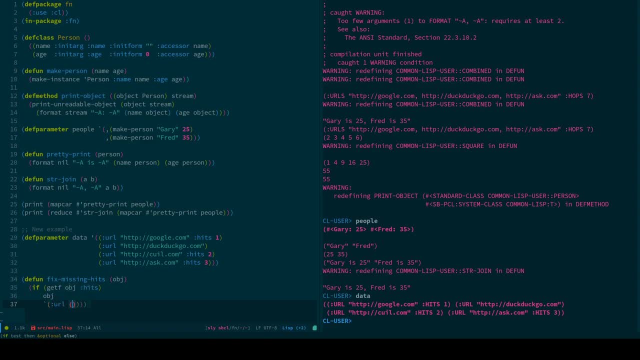 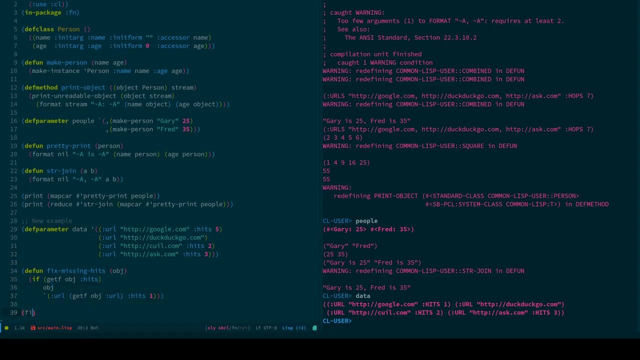 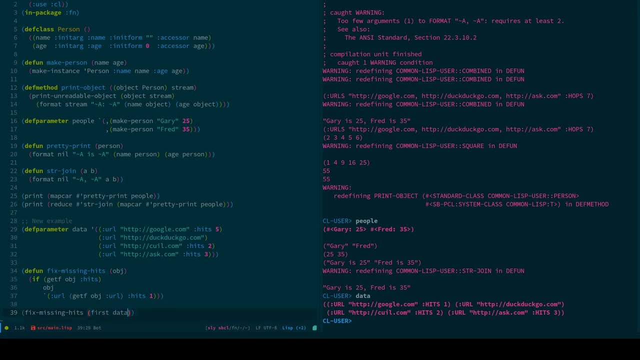 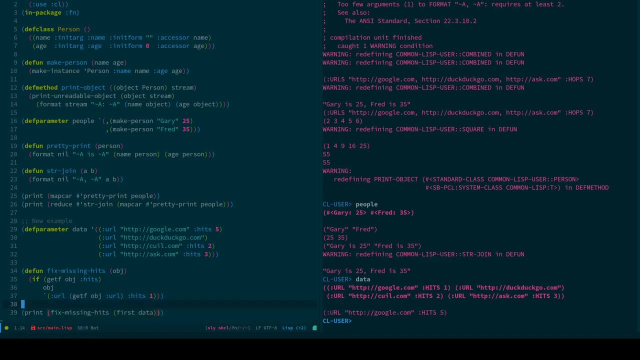 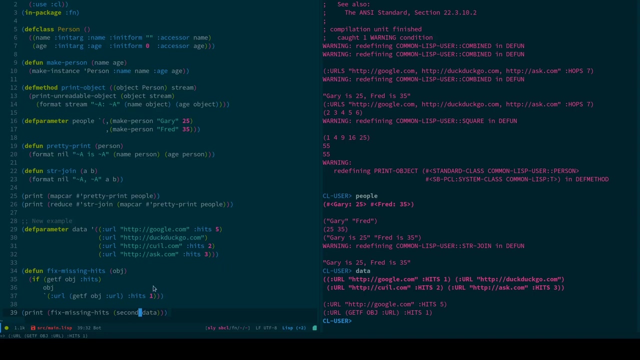 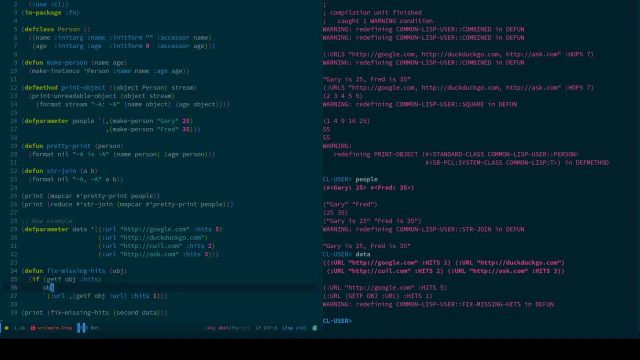 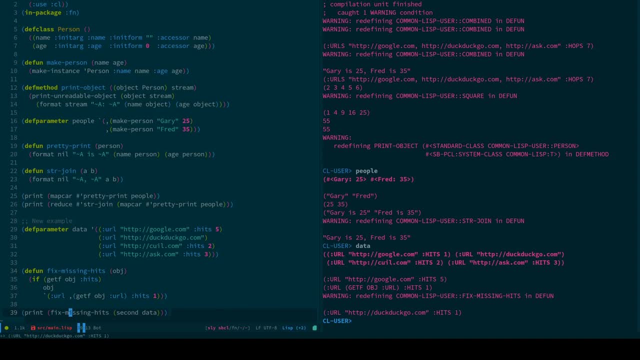 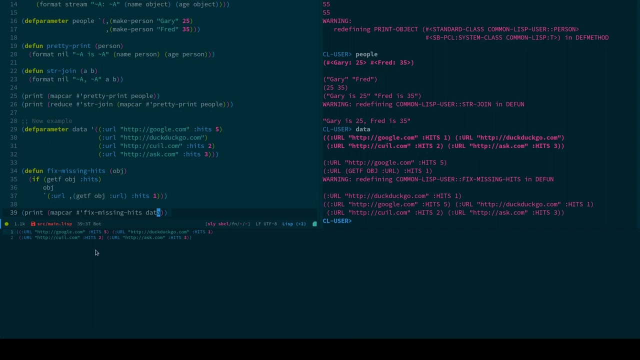 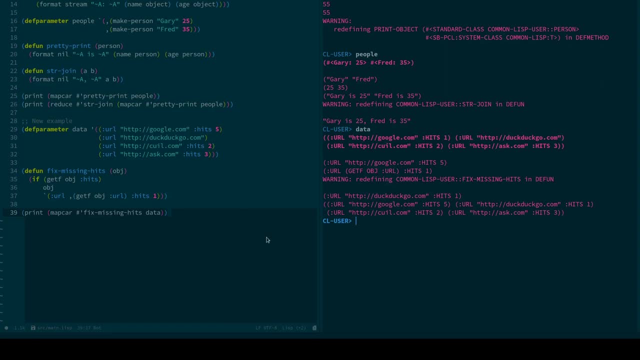 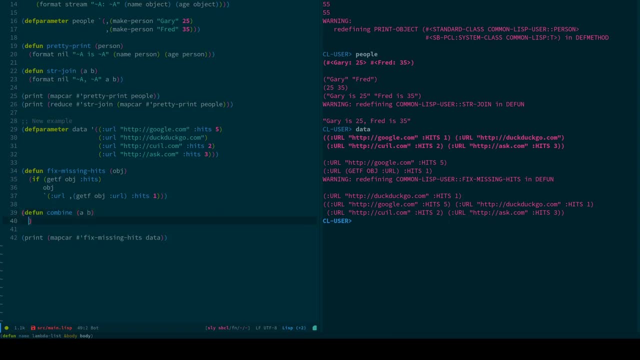 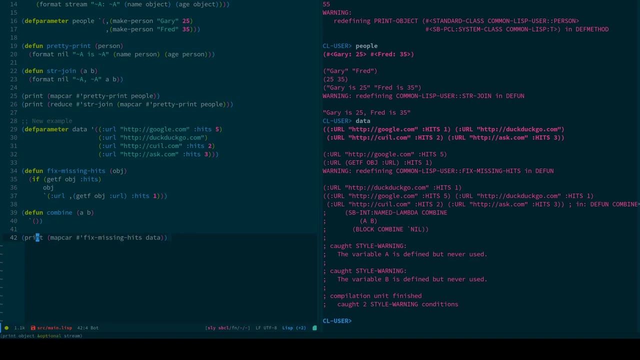 and because we're going to use this as a reducer- it takes an a and a b- we are simply going to return a list here. this is going to be an empty list and we're just going to prove that it works, because i am a big fan of making sure everything is plugged in. 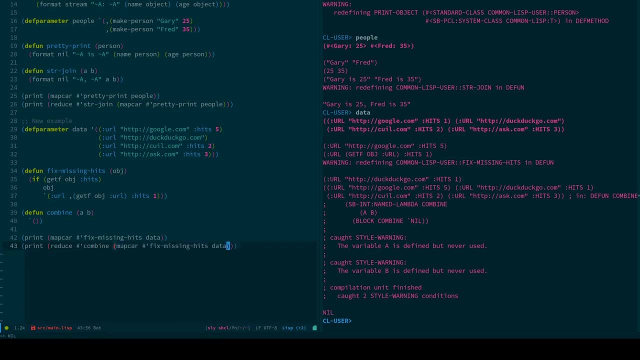 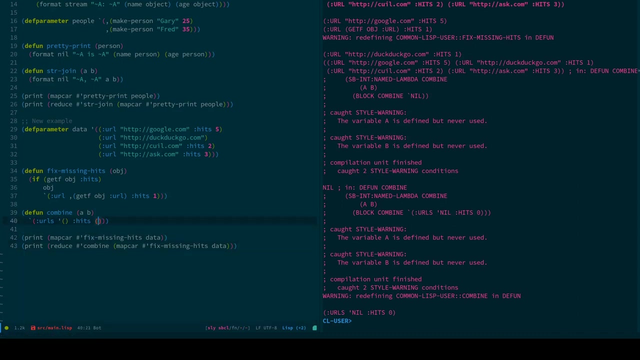 and we fix things up as we go. so, yes, we got nil. that is exactly what we want. so we want to return this urls and we're going to say empty list. we're going to say hits zero, cool, so let's start with the hits. we want to return the result of summing um, get f. 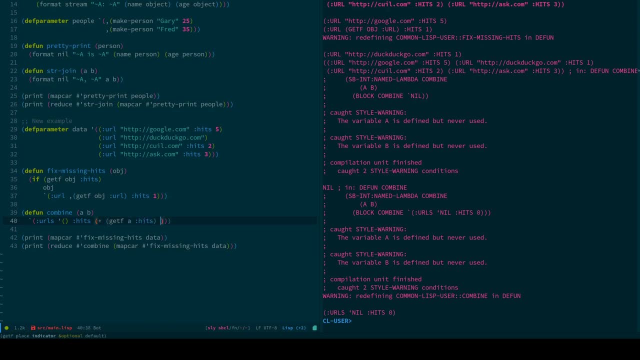 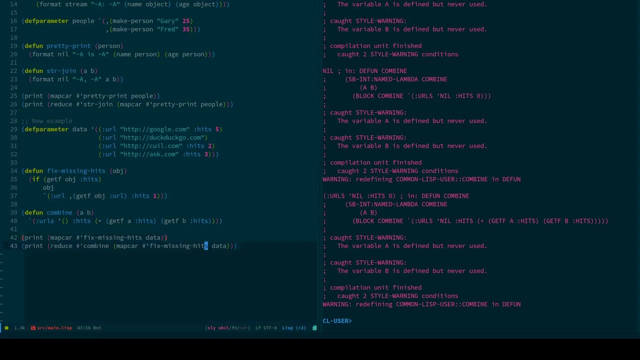 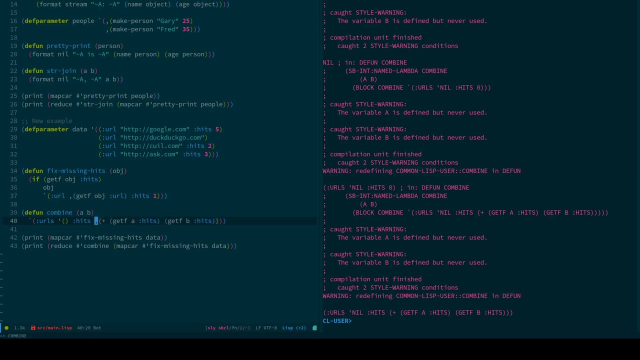 a hits and get f b hits, because a will get accumulated to and the way that works together, we should put a comma there, of course. my bad, there we go. so we've got hits 11.. so five plus five plus one, that is 11.. so that is correct. 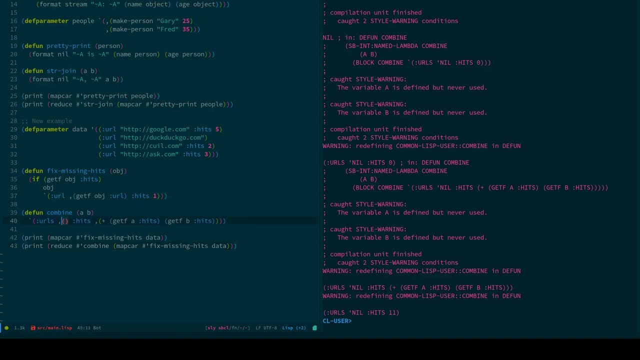 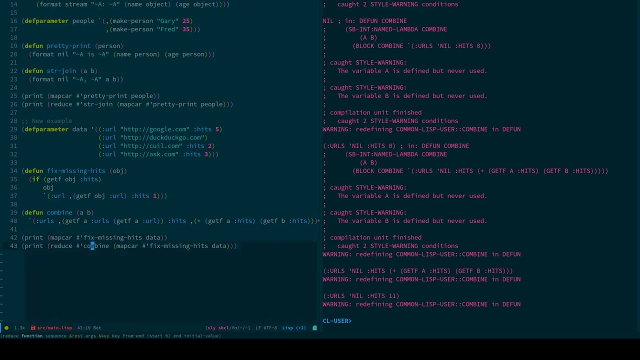 what we then want to do is we want to say: um, get f, you are a urls, or get f a, you r l, and that is us using the default behavior of getf, where we can supply a default arguments. if there's no URLs in this P list, we can then get the individual. 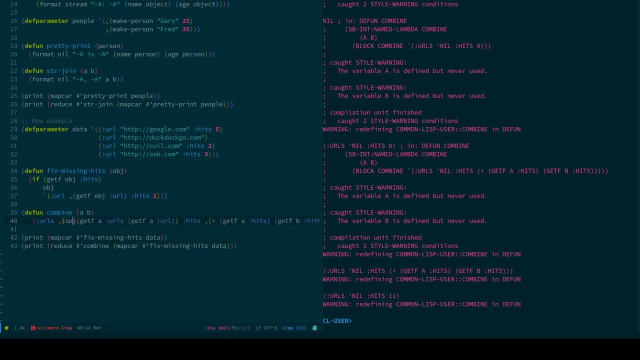 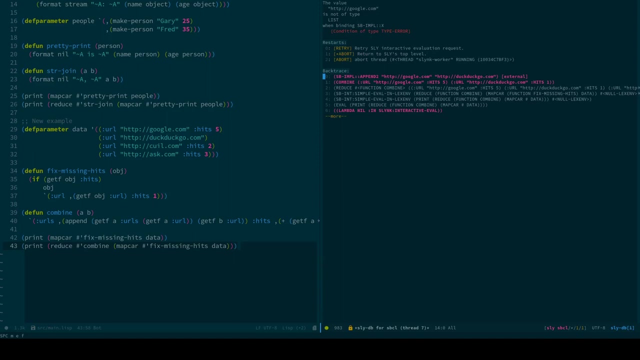 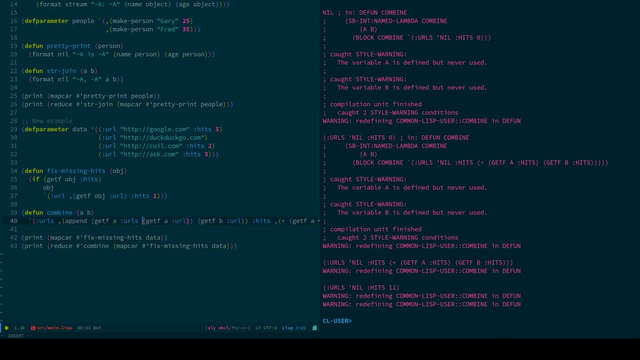 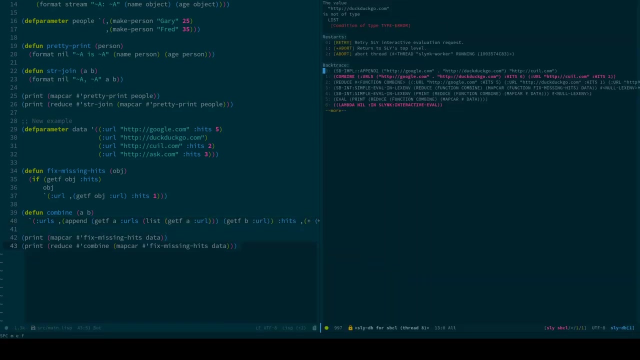 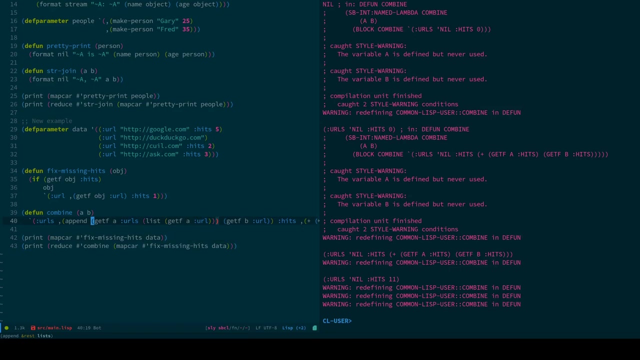 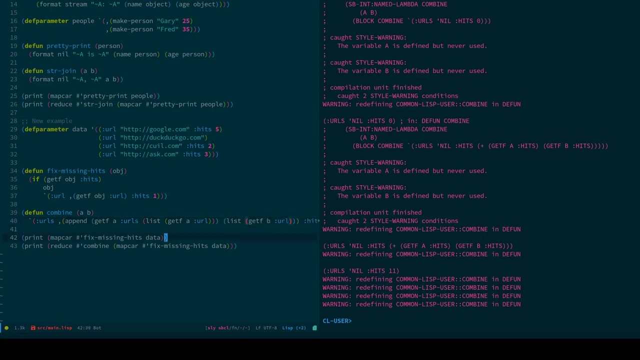 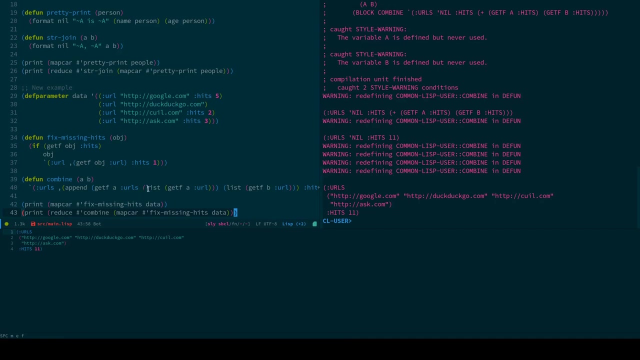 and what we then want to do is say: append this with the getf, the URL. So if we redefine that, we have an error, say list. so there we go. I just got my- my nomenclature a little bit wrong there. so yes, We are appending. 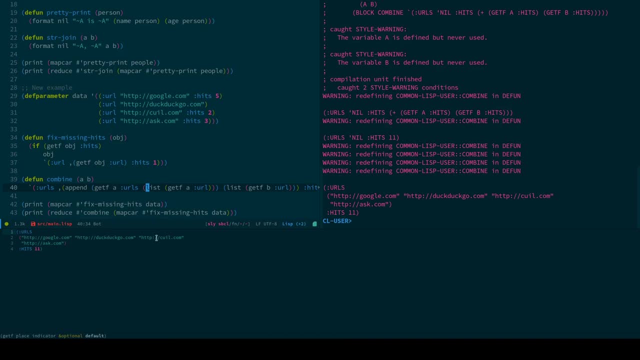 all of the URLs together. so we get thisgoogle goql ask and then we say: between them, there we go, were 11 hits. So that is us taking a list of P lists, so a list of lists here, and we're combining that all down to a single P list, Moving through map to turn each of these into. 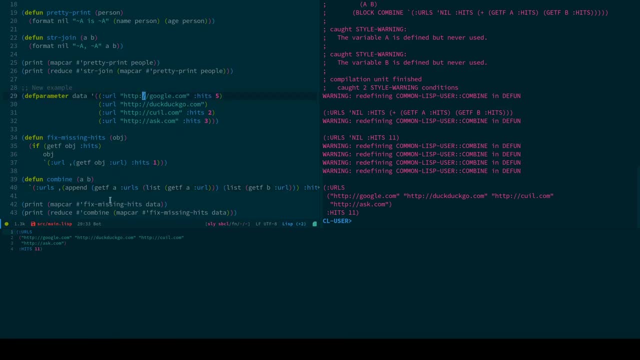 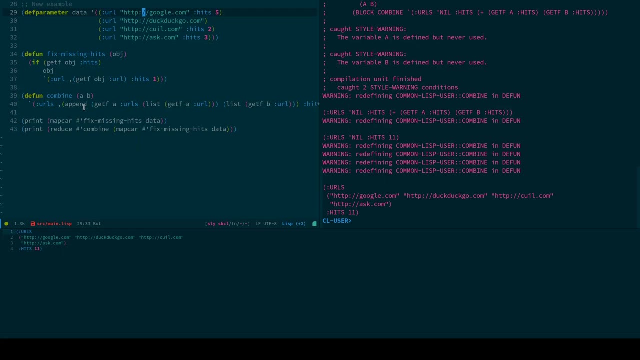 corrected data so they all have a value somewhere, and then combining them all down into a single P list by adding and changing, by returning a new P list every time. It's a rather recursive way of thinking about it, or rather, it's a very functional way of. 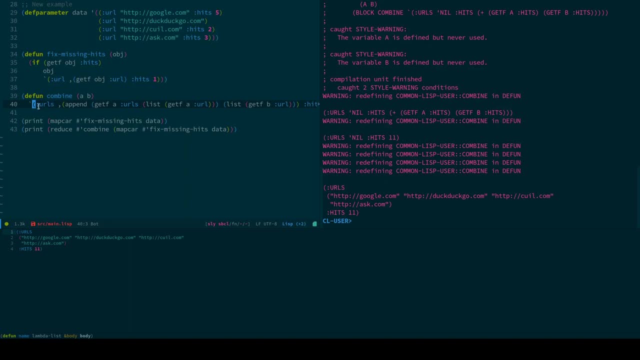 throwing away the initial object and just pulling bits out and rebuilding it. but you see this a lot in the closure world, So that's kind of cool. I want we can use the behavior of getf to return a default if there is not one, so on the first time we're going to return. 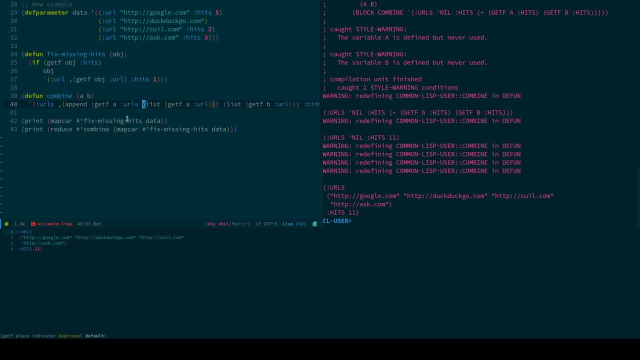 to return the list of the first one and that will build a list which we can then pull back out. and then we get the list of URL here and we're just going to add that together, because when we append, we need to append lists, just like so. 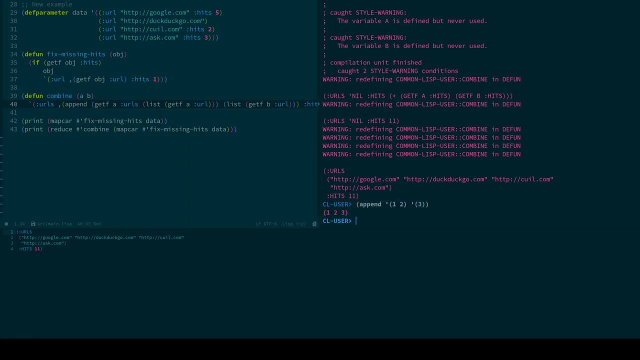 otherwise we would get a con cell with one, two and dot three, so everything had to be in a list of there. so that is an example of how map and reduce can be combined together. this, although it's a stripped-down version. this was actually practically pulled out of a code base I was previously working on. where we can. 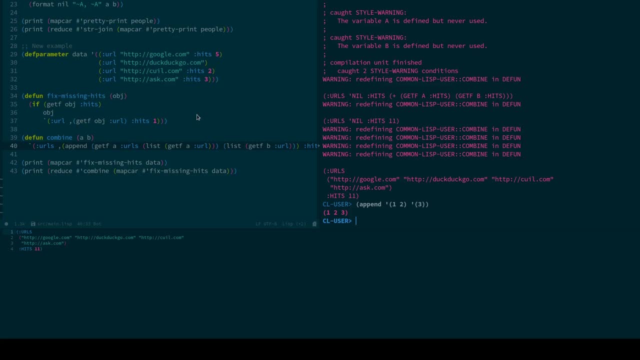 use map to fill in the blanks in some data that might be missing, then we reduced that all down to something that we we cared about. so the that is it. that is a very, very brief look at how map and reduce can work together. I'm keeping it brief this week because of the problems that I'm having.